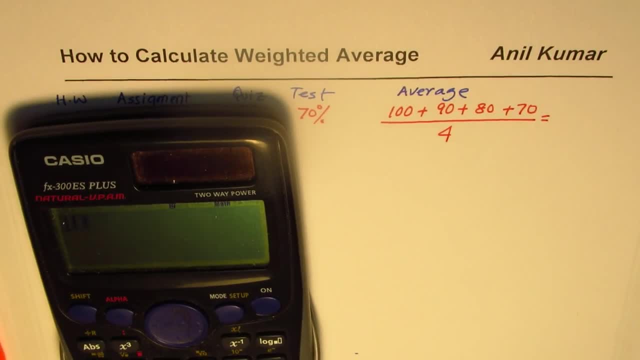 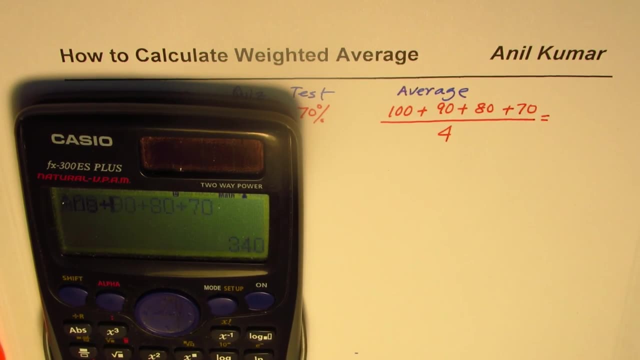 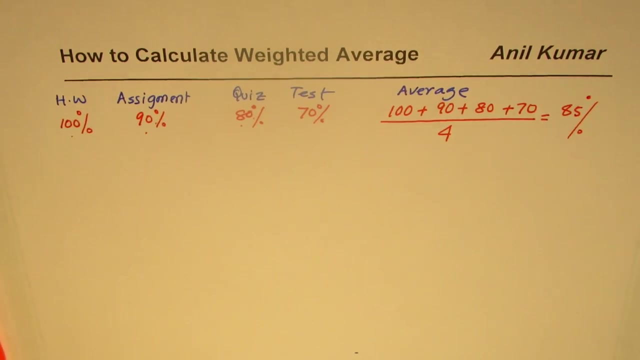 answer. so let's do it so. we have hundred plus ninety plus eighty plus seventy, that is equal to three hundred forty divided by four, that gives us average which is eighty five, and let's put percent to it. so eighty-five percent is the average and you can clearly see that this average eighty-five is kind of in the centre. do you see that so kind? 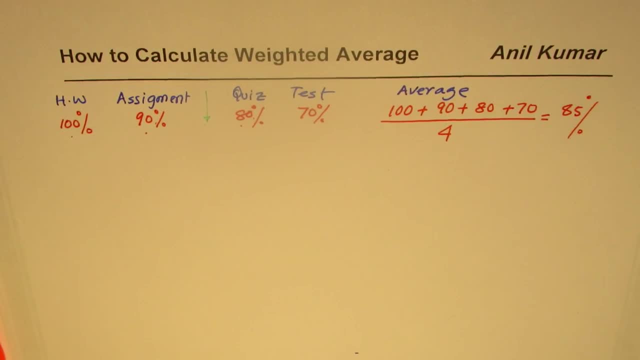 of here, somewhere, somewhere here, ok, eighty-five. So this happens when all these tests, homeworks or assignments are at par right, So they have the same weight, but normally you'll find they don't have same weight. Now what does that weight means? 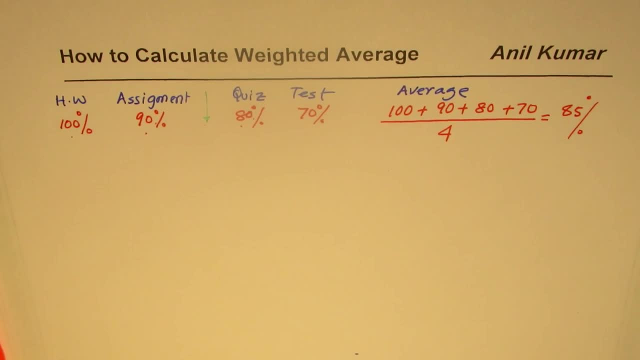 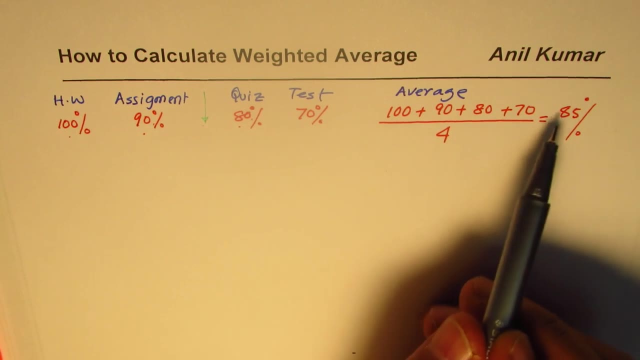 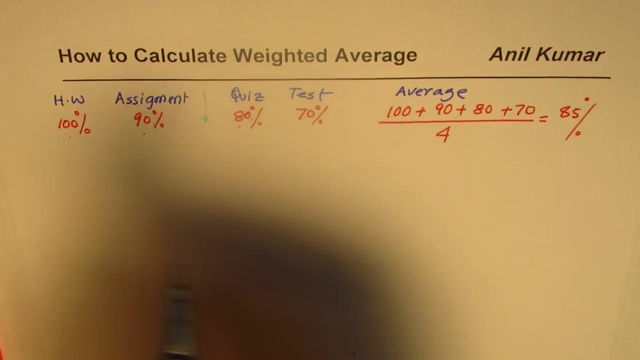 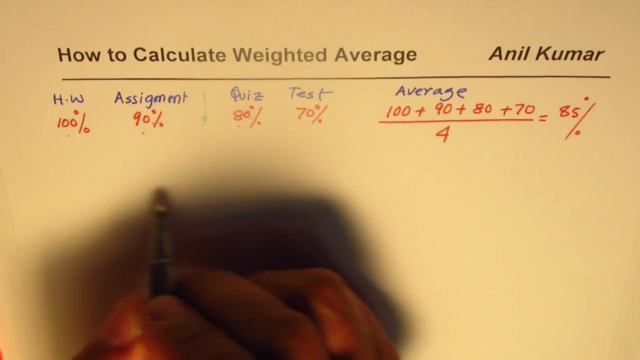 Weight really means here that what we are saying that they're all equal. How Let's say what is this like 85%, right? So we divide everything by 4. That means kind of quarter. So what we are saying here is that everything has quarter, quarter, quarter, quarter to add up to make a full. 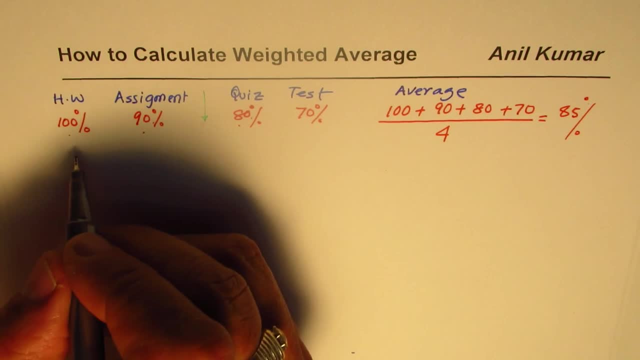 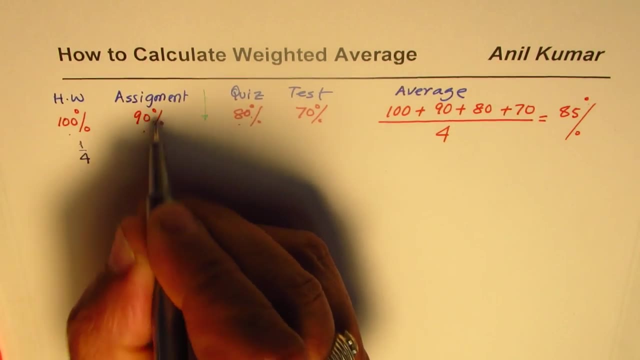 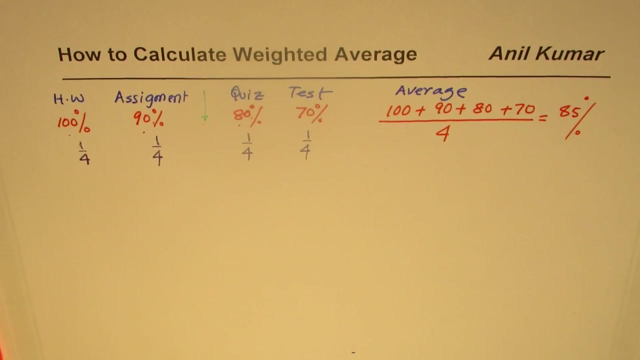 So the weightage which we'll introduce further is: it is like one-fourth of the marks, one-fourth of the assignment, one-fourth of the quiz and one-fourth of the test is being added To find the average. well, let's do that. 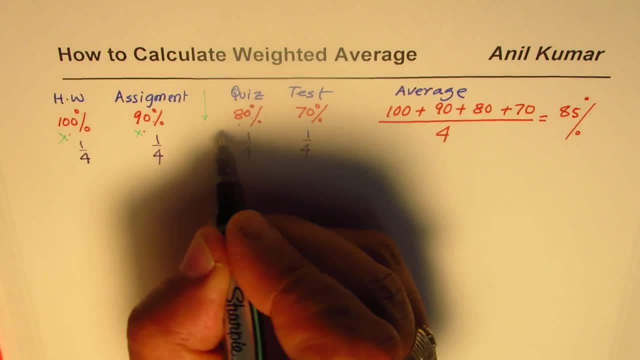 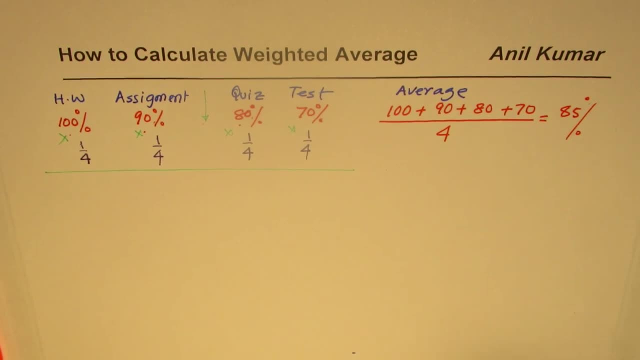 So if I multiply these two, kind of let's say we multiply these two, see what do we get. Let's multiply. So what is one-fourth of 100?? So we'll do one-fourth of each and then see if we get the same result or not. okay, 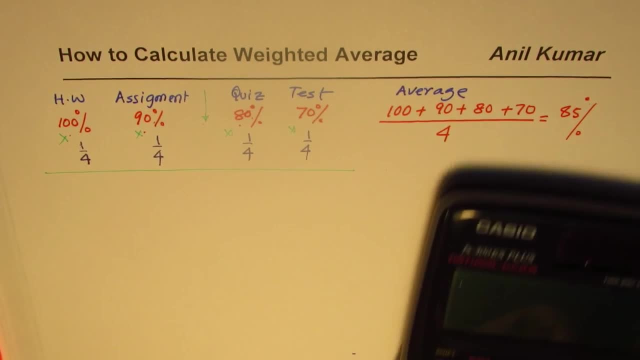 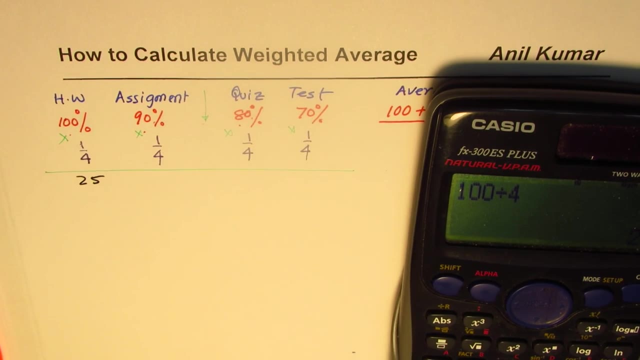 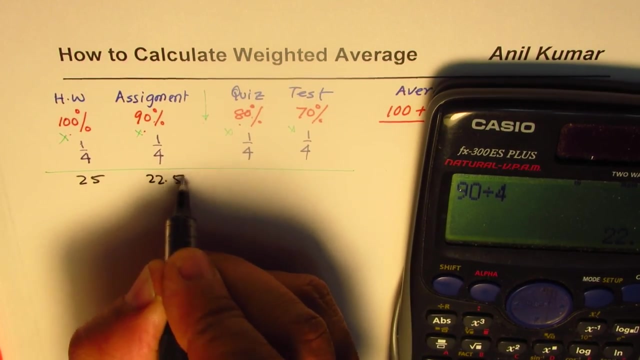 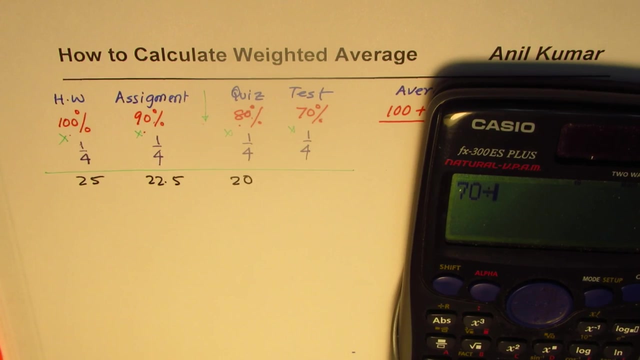 So let's find out. So what we get here is: one-fourth means 100 divided by 4.. One-fourth is 25,. we get 25 here. 90 divided by 4 is- let's write in decimals- 22.5, 22.5, 80 divided by 4 is 20, and 70 divided by 4 in decimals is 17.5, 17.5.. 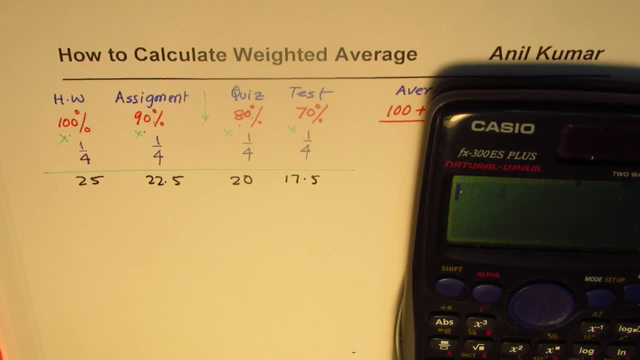 If I add them, what do I get? So what I have here is 25 plus 22.5 plus 20 plus 17.5, all this is equals to again the same number: 85, right, So we get 85.. 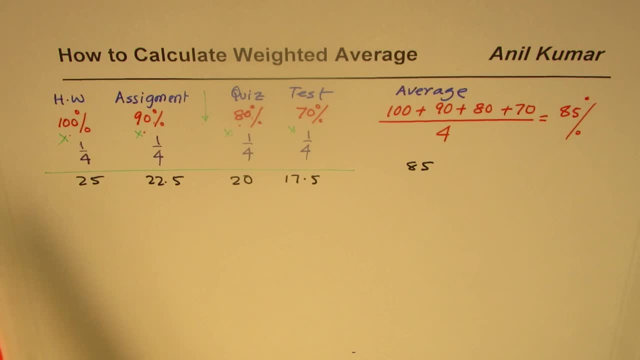 Do you see, We again got the same number. So when we say that they are at par, then we say they have the same weight. And again, multiplying the weight by the marks, we get a number which, when added, gives us the average. 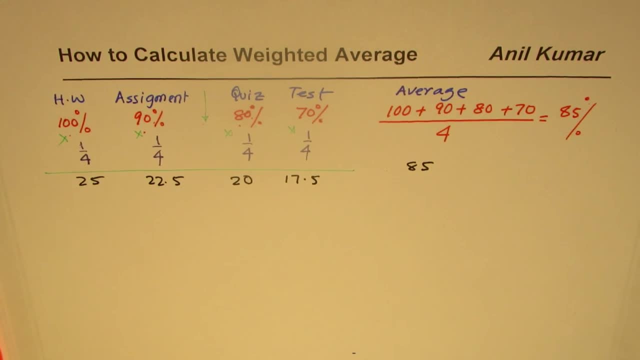 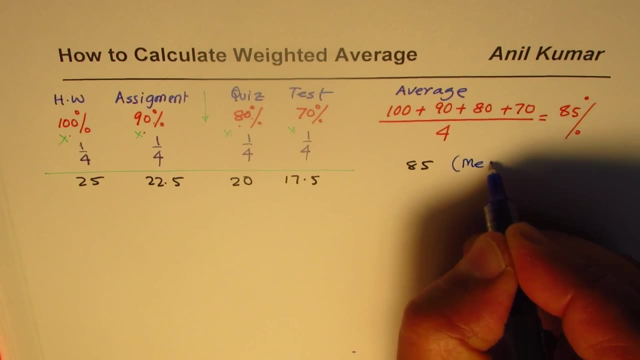 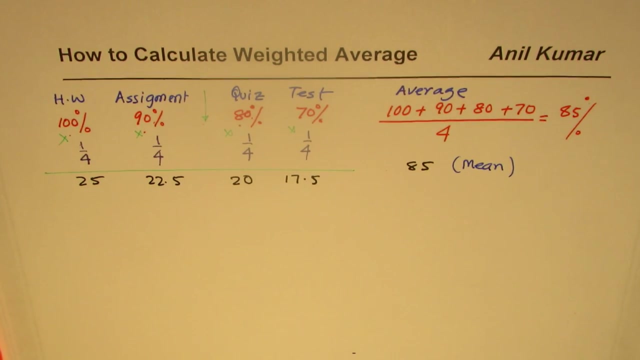 You understand the concept right. So that is what It is when we take up normal averages or the mean right. So at times we also call this as mean right, Mean value, average value, right, And you will always see that mean value is somewhere in between, correct? 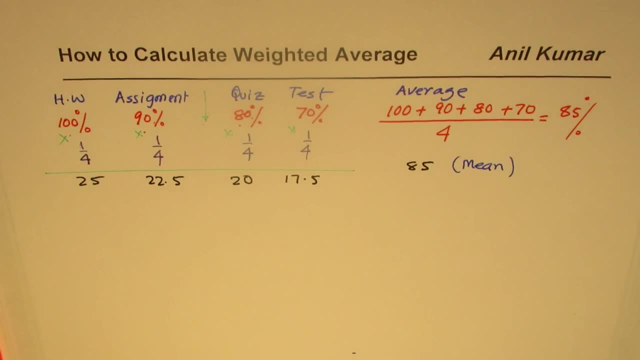 Now, practically, you have always seen that their weightage is not the same. No one is going to give same weightage for homework as for the final test, right? It doesn't make sense. So let's say, instead of writing: 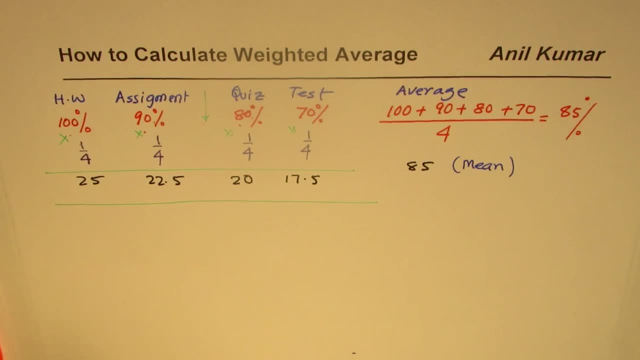 Let's say, instead of writing in fractions, we'll take up this in decimals. okay, Quarter could be written as 0.25, as you can see right, So that is 25%. So, which is same as we could write this as 25%. 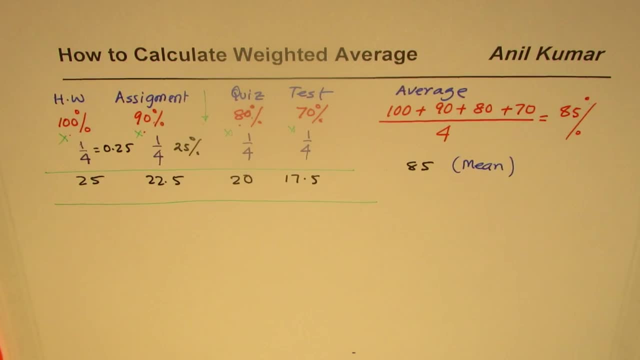 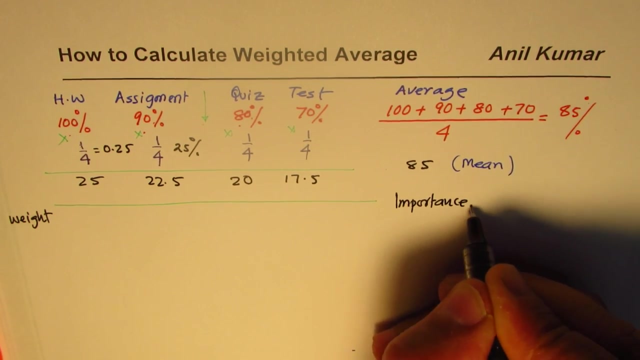 Both are same things, right? So what I will do this time is we'll write percent weight, So we are using the word weight. now That means importance is different, right? So we are writing weight or importance Right, Or significance, right. 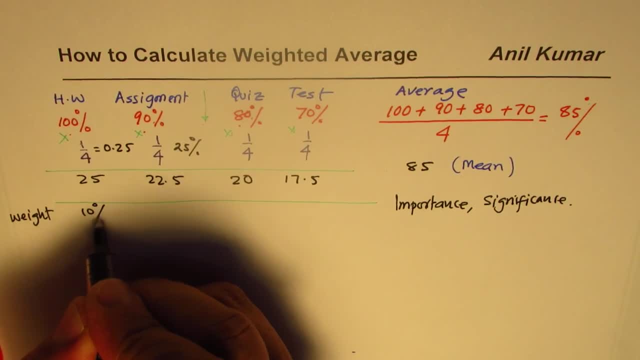 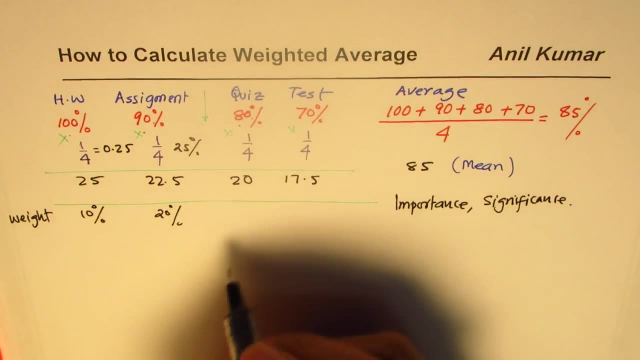 Okay, We say for homework it is only 10%, right, And for assignment we'll give 20%. It's a take-home assignment Quiz. let's say we give them 30%. So how much we have already allocated? 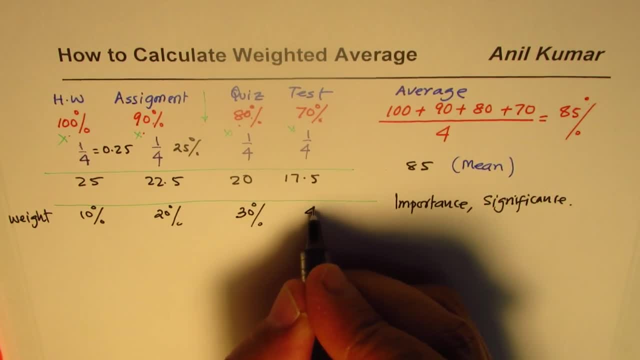 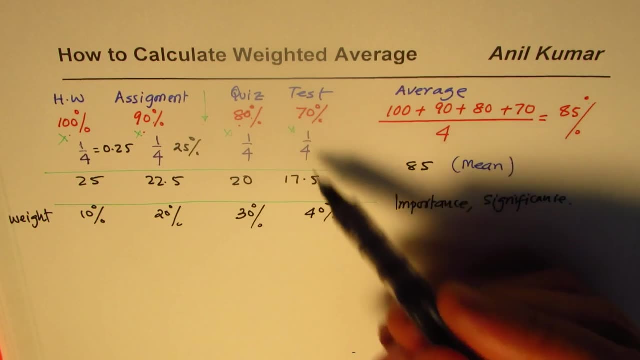 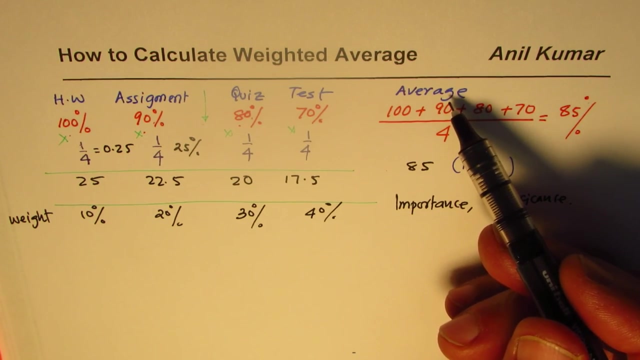 10 plus 20 is 30.. 30 plus 30 is 60.. We're left with 40%. Now all have different weight or importance For test. it is 40%, not 25%, as it is when we talk about normal, mean or average. 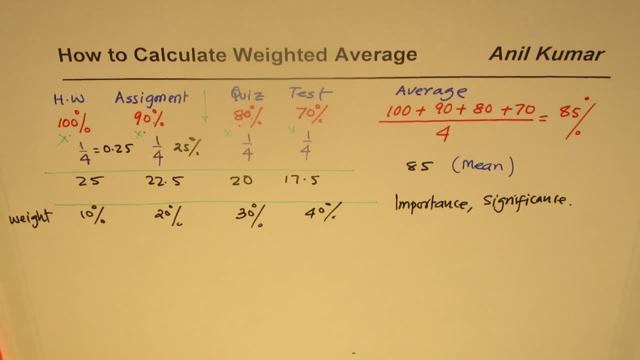 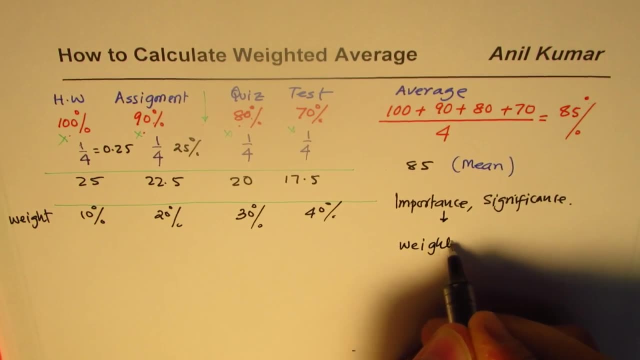 But homework is only 10%. Now how to find this weighted average? So now we are talking about weighted average. Do you understand? Considering the importance of each right? So which is different? So we are talking about weighted average. Let us see how to figure that out. 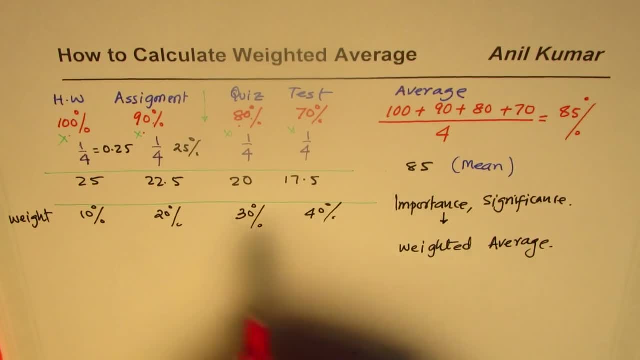 First step here is better to write this percent in decimal. So we are considering decimals so that we can straightaway multiply. It could be fractions also, But decimals is the standard way. So 10% means 10 out of 100, right. 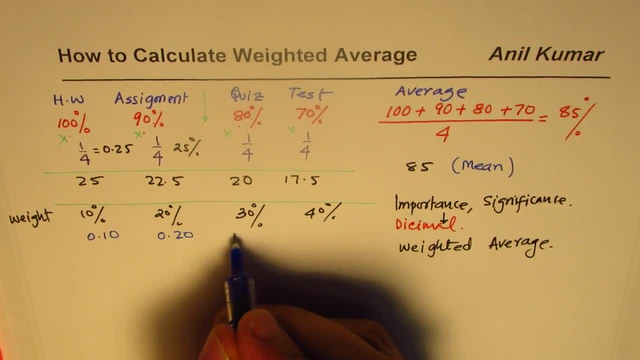 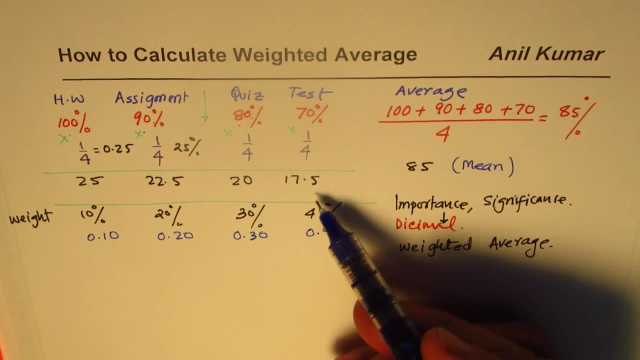 So it means 0.10.. This is 0.20.. Decimal equivalent for 30% is that, And for 40, 0.40.. Now, as we did earlier, we'll multiply the marks with with the weight. so this is weight per in decimals that. 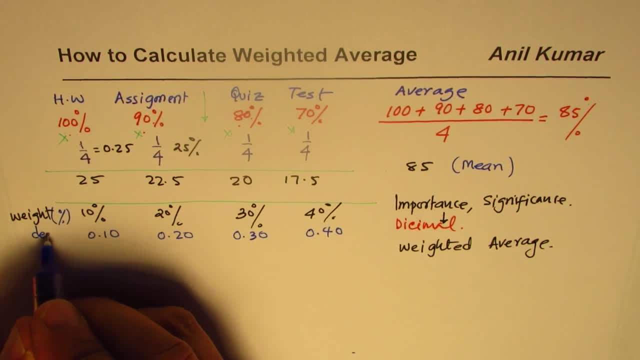 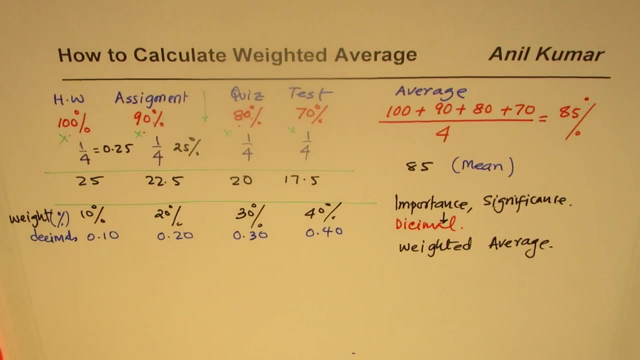 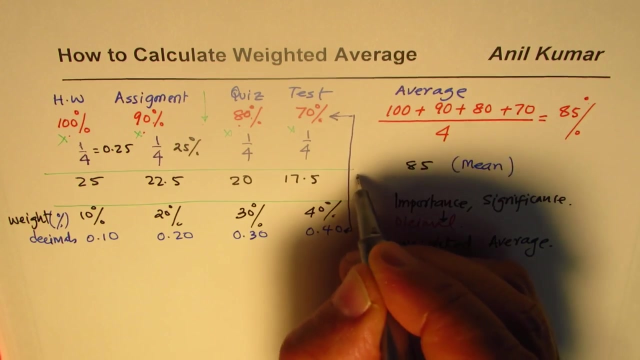 was weight in percent. right now we have it in decimals. so what we will do now is multiply the marks obtained with. these are the marks obtained, right, these are the marks obtained. we are going to multiply with the weights. we'll do times operation on this and write down. so what? 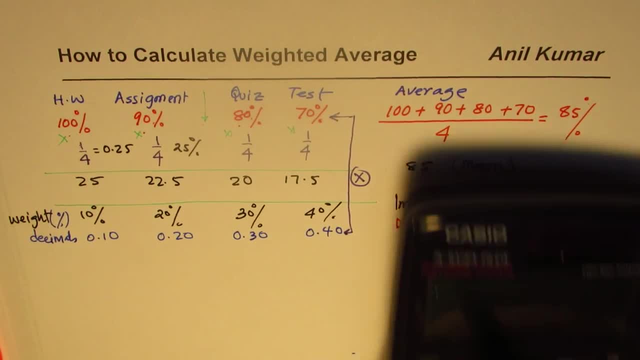 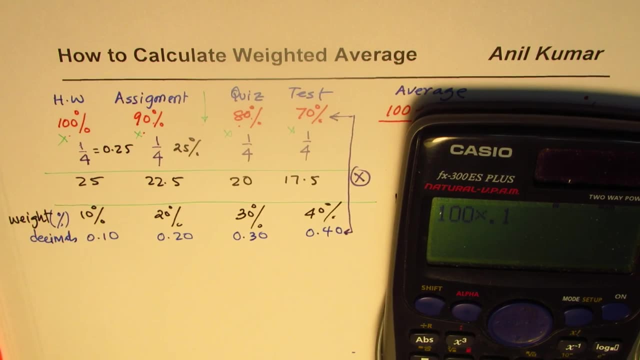 do we have. so let's multiply each. so it is hundred times point one. so it is hundred times point one equals to ten. so we get a mark here: ten, ninety times point two. ninety times point two equals to eighteen. and then we have eighty times point three. eighty times point three is equals to 24. 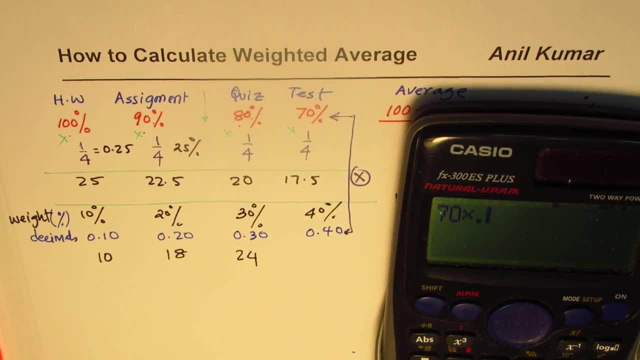 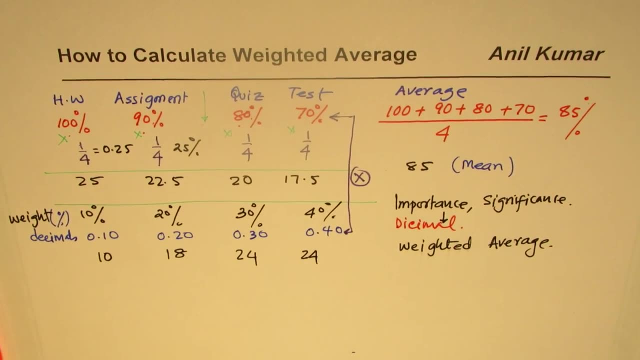 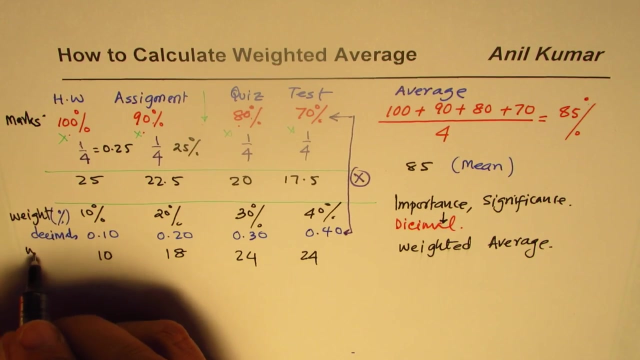 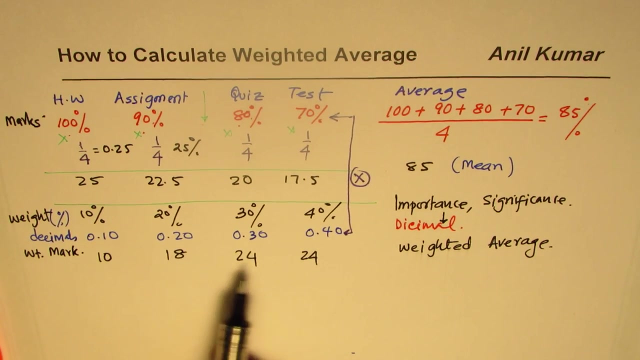 and then we have seventy times point four equals to twenty eight, so we have twenty eight. so these are weighted marks. so these are weighted marks. those were our marks, right? these are weighted marks. so let me write weighted marks. how do you find the average? to find the average, these are four different weighted 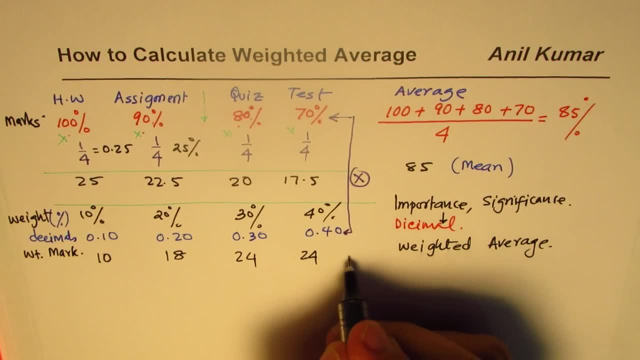 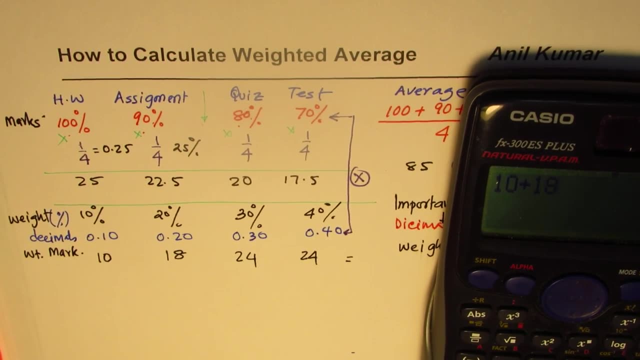 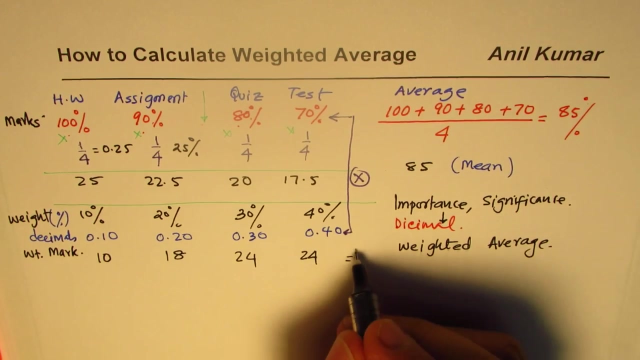 marks. right, we'll just add them up, right? so if you add them up, what do you get? so let's add them up, so we have 10 plus 18 plus 24 plus 24, and that is equal to 76, so we get the number, which is 76. 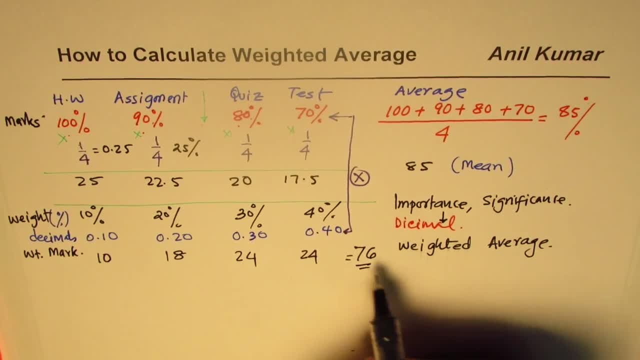 do you get it? as you can see, the 76 is much different than 85. our weighted average is much lower, since the importance of test, where we did not really score much, is higher. so we got a lower weight age right. so so that's what happens. so what do you see here? is that the number now? 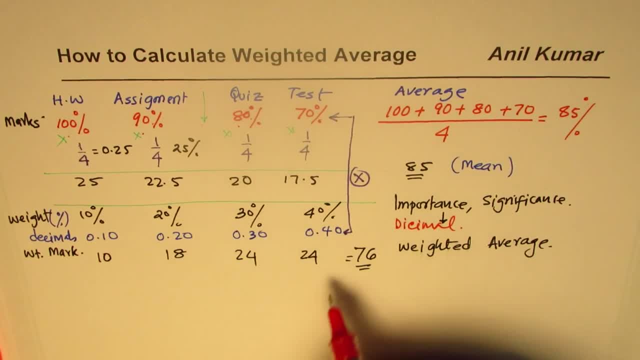 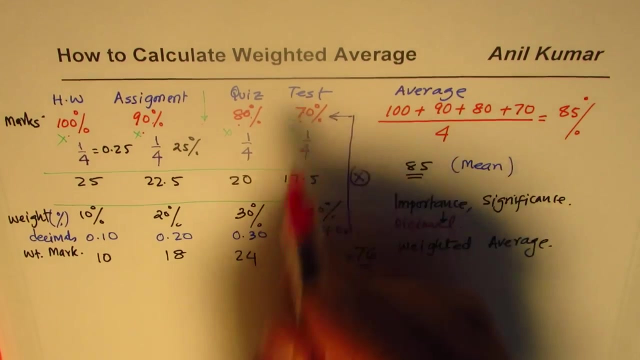 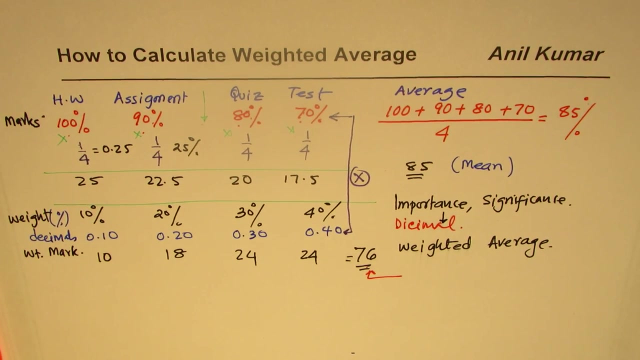 instead of falling right there in between, it moves more towards seventy percent, the original, whose weight is more right. so this 76 is closer to seventy percent. do you see that? so it is closer to seventy percent, rather than homework and assignment, where the school was much higher. you get an idea. so so that is what it shows, if weight is more, if 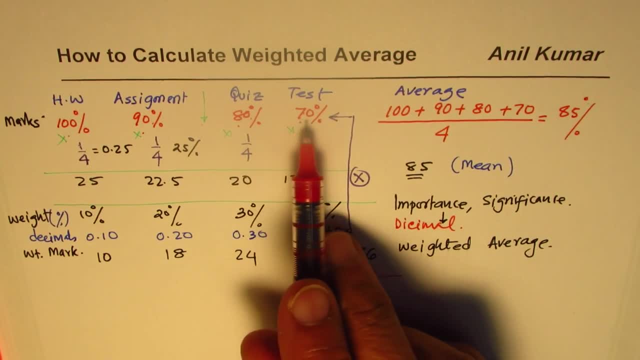 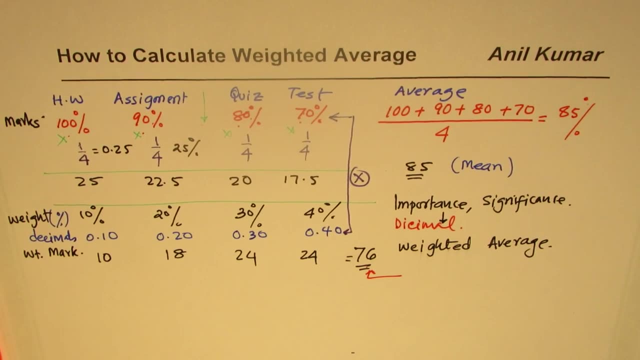 there are more numbers, then the average moves towards higher numbers. so it is 76, much lower than previous average, closer to the marks which are highest weightage marks, correct? so that is how it is. so I hope you understand the concept and for you let me give you. 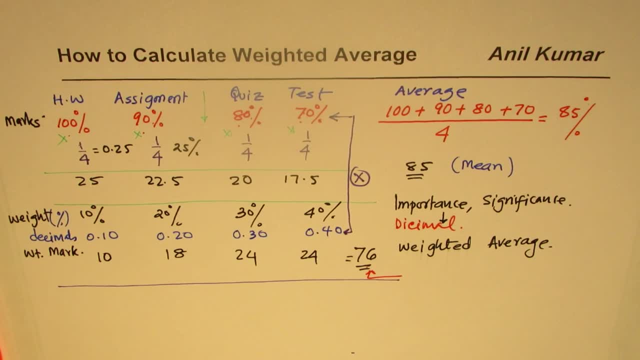 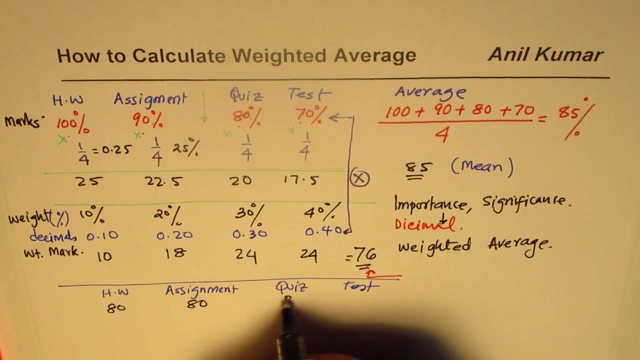 a practice question. so let us say- this time a question for you- that we have homework, assignment, quiz and a test. the marks obtained are, let's say they are same. let's say, let's say, let's say, in homework it is 80, assignment is 80, quiz 80, test 80.. but the weightage, these are the marks obtained. 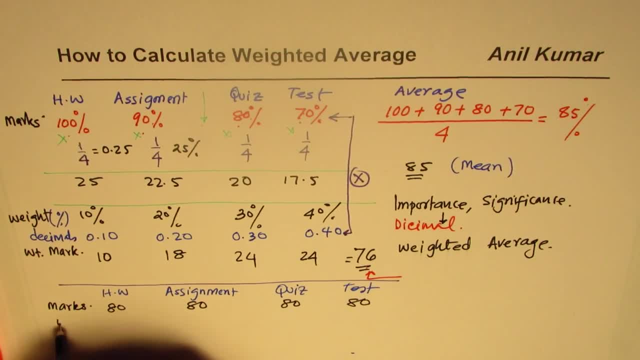 right, these are the marks obtained, and the weight is, as we used here, 10 percent, so we'll write in decimals. let's write 10 percent, okay, 20 percent, 30 percent and 40 percent, right? in this case, what happens is the average 80. let us calculate. so calculate what happens. you need to multiply these. 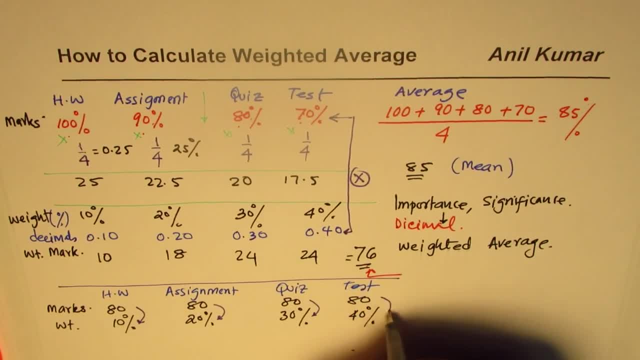 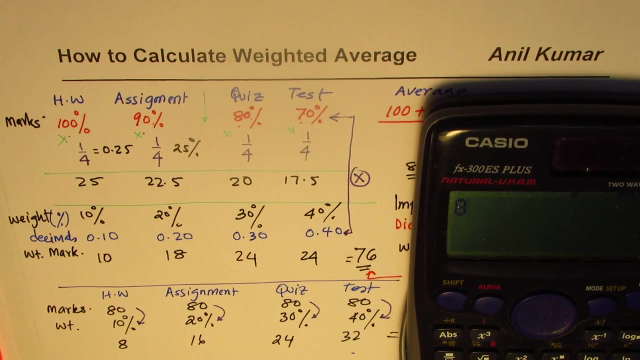 two and then add the average is correct. so these are the weighted averages. let's multiply 80 with 0.1, so what do you get? 10%, 80, 80 with 0.1 is 8 for you. 8 times 2 is 16, 8 times 3 is 24, 8 times 4 is 32. let's add them up so we get 8 plus 16. 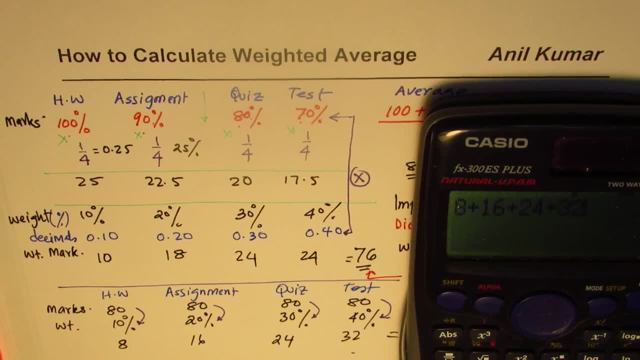 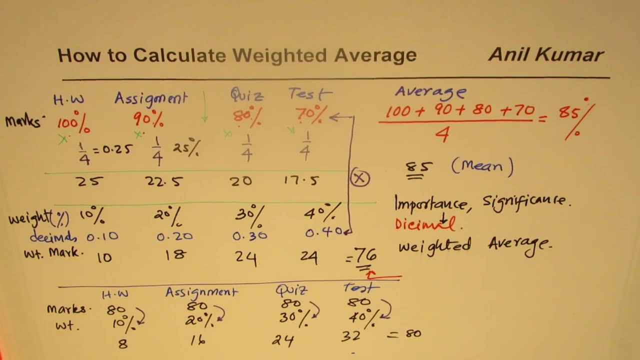 plus 24 plus 32 equals to 80. do you see that? so we get a number which is still 80. so if you get same marks, it is going to pull towards the marks which has highest weight. weight is same, right. therefore the percent remains the same. 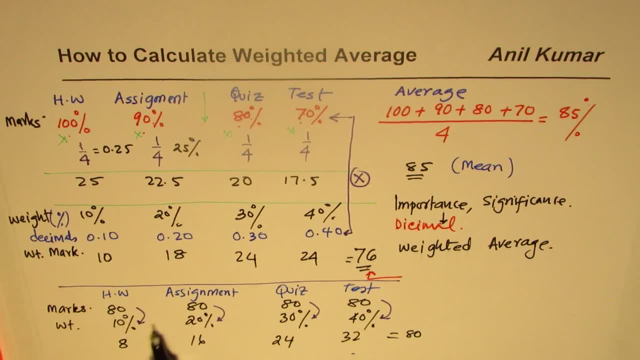 so in this particular case, the weighted average becomes similar to the mean, the average correct, because the marks were same. do you get an idea? okay? so now a question for you. if I change the marks all together and if I say that my marks for homework, let me. 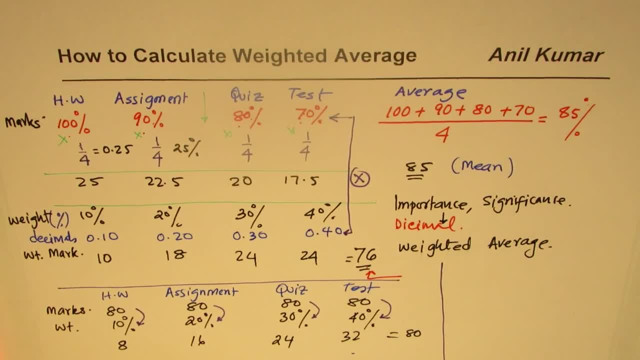 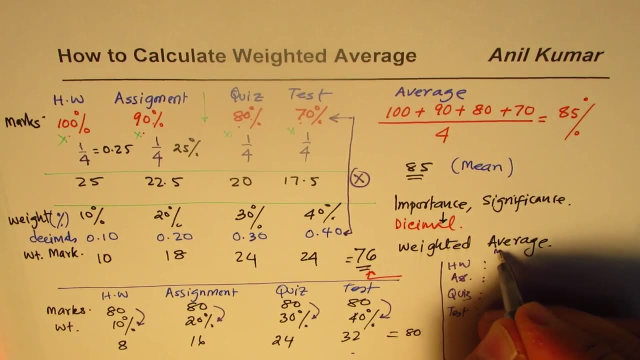 write down this question here for you. where will the weighted average be? so I'm saying homework, assignment, quiz and test, right, so let me write down the marks and their weight. age, right, so we'll write down the marks and weight. okay, marks are, let's say, homework 90, assignment: we have 60. 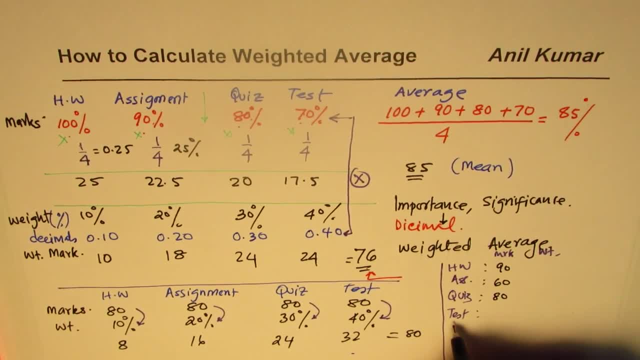 quiz we have 80 and test we have, let us say, 95, and the weight in this particular case is, let's say, 100%. I mean, sorry, 10%, 20%, so that means 30, and let's say this is 30%, 60, 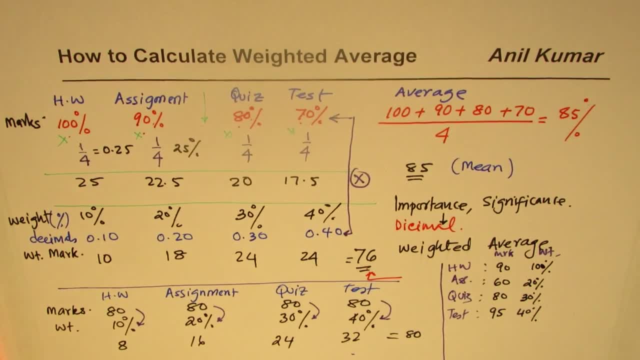 let's keep 40%, same weight as we have taken in our example. what do you think will be the weighted average here? so the question is: weighted average will be closer to which value? it will be very close to. closer to 90, 95, right, because 95 is the marks for highest rate. so just multiply them right, and find the.